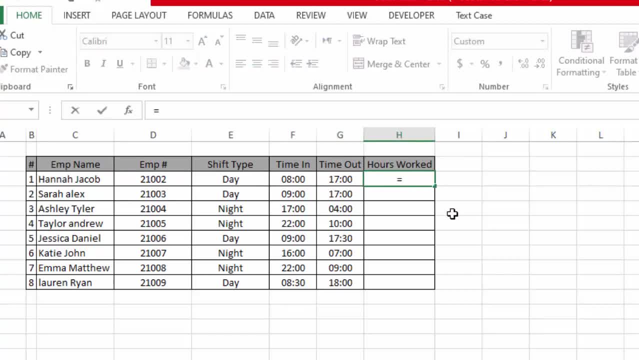 worked actually right. so for that, what we do, we simply minus time in from time out. so for that, what we do: equal sign time out minus time in, and this is the actual hours worked by an employee. we just drag it down and you can see here, this is the error that i'm talking about. 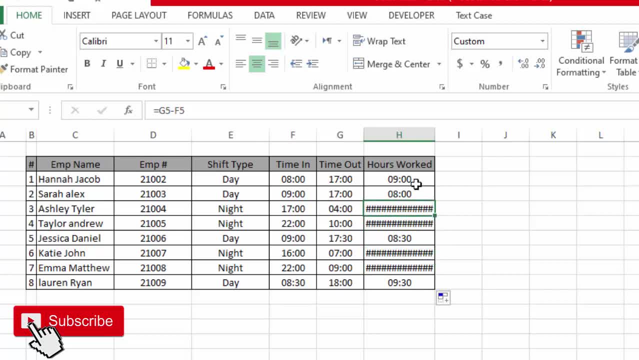 the most of the people face this problem or this error. you can see this is simple, of 17 minus 8. this is simple. 9, 17 minus 9, simple, this is it. but here you can see this is error. why the thing is behind this error is that actually the time behaves same like numbers. you can see here, if we minus 17 from 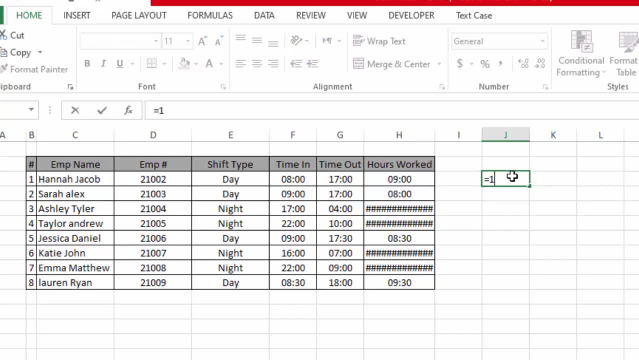 8, 17. sorry, 17 minus 8, this is simply 9. but here, as this employee is working on ninth shift, mean he's started working on 4 am before, even before morning, and he stopped working on 17, that is actually 5 pm. so, as you know, 4 is smaller than 17. so when we what we do, 4 minus 17, the answer is in: 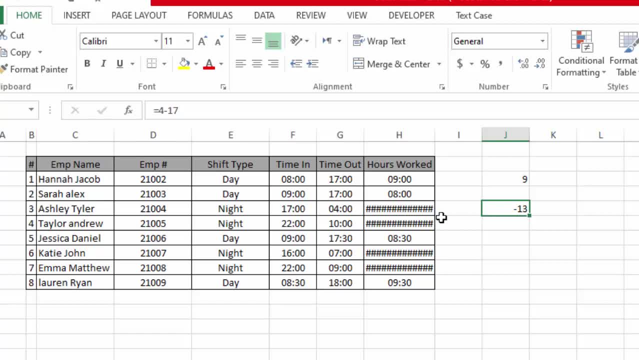 negative, and we know that time can never be negative, and when it answer here is in negative, it shows us error, because we are trying to calculate time right and time can never be in negative. so what is that solution here? actually, the thing is, one thing is here that mostly people when face this problem, they just 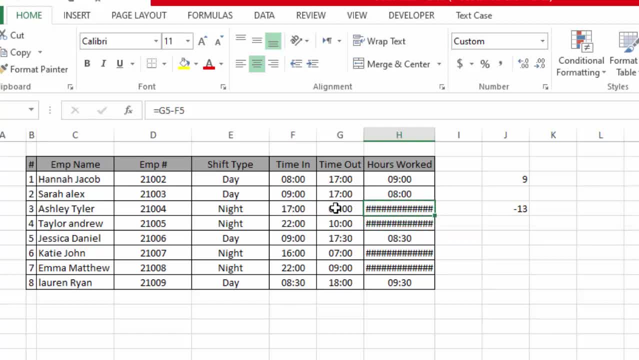 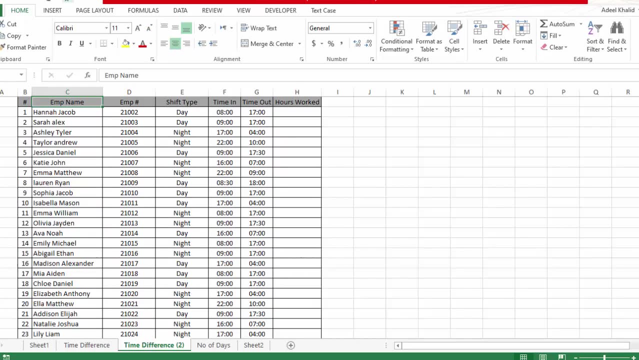 work manually. they just calculate manually and just. they will write here 11 hours. but here this is okay. here we have very small amount of data. but what if we have a lot amount of data? you can see, here here we have more than 250 employees. so if we try to use the same thing, if we do timeout minus. 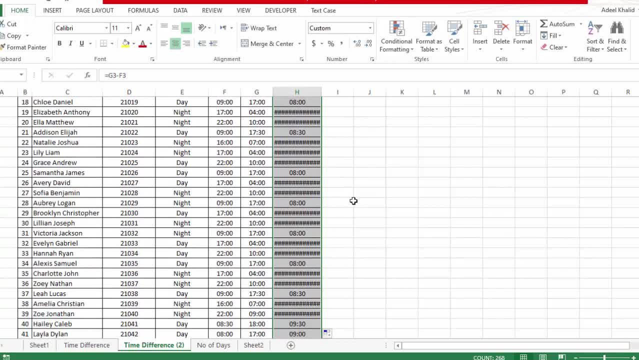 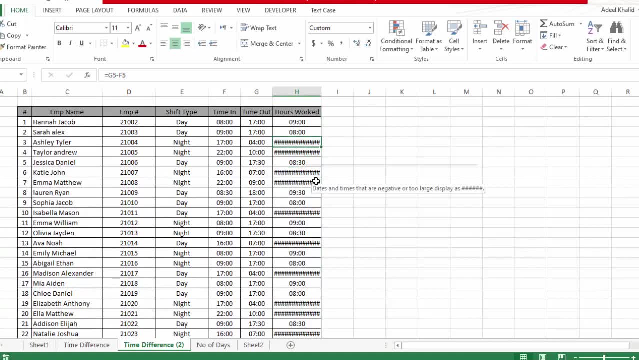 and just we drag it down. and you can see here, here we have a lot of errors. wherever an employee has night shift, we have error, so we cannot work manually. this will take a lot of time, right, so we need to find out any solution for this. so what is solution for this problem? solution for: